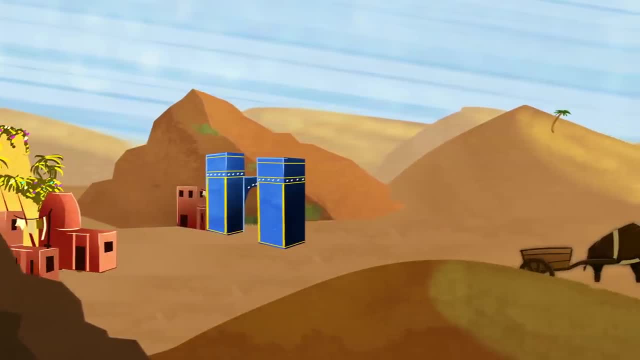 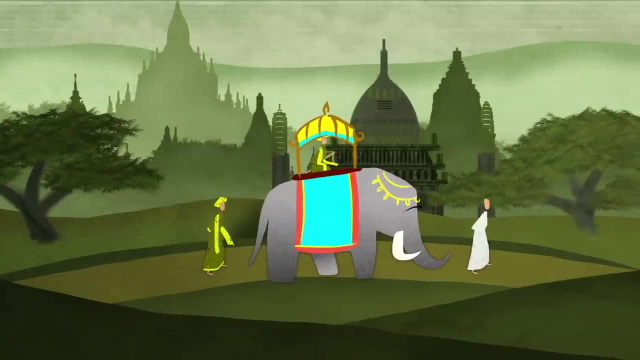 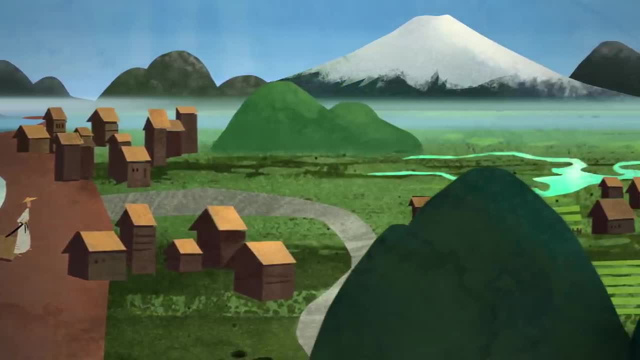 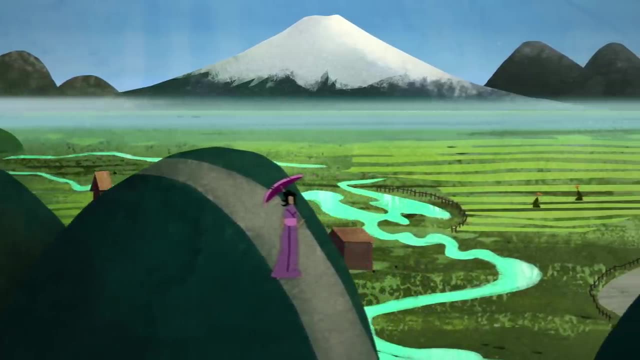 were drawn from the countryside to the cities as more jobs and opportunities became available. If you think modern cities are overcrowded, you may be surprised to learn that some cities in 2,000 BC was popular with famous business organizations and business institutions. 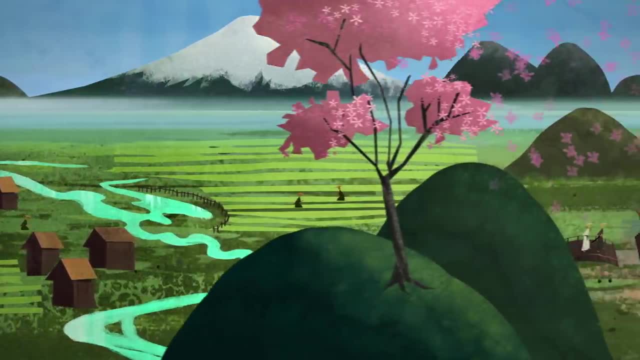 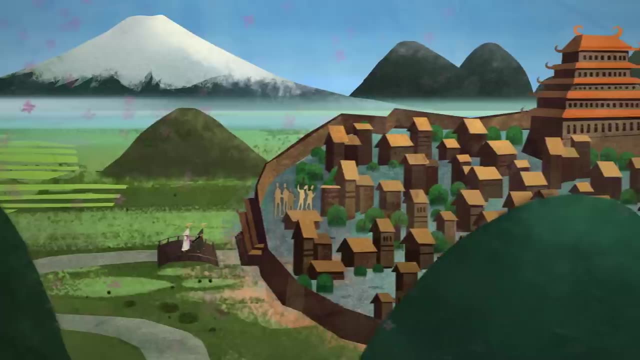 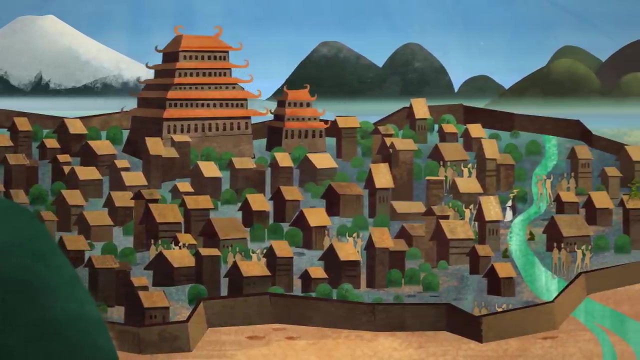 had population densities nearly twice as high as that of Shanghai or Calcutta. One reason for this was that transportation was not widely available, so everything had to be within walking distance, including the few sources of clean water that existed then, And the land area of the city was further restricted. by the need for walls to defend against attacks. The Roman Empire was able to develop infrastructure to overcome these limitations. but other than that, modern cities as we know them didn't really get their start until the Industrial Revolution, when new technology deployed on a mass scale. 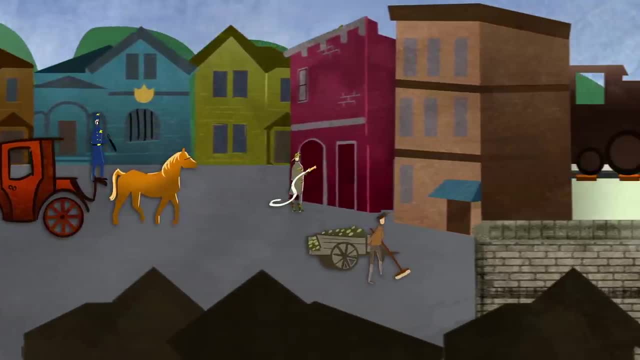 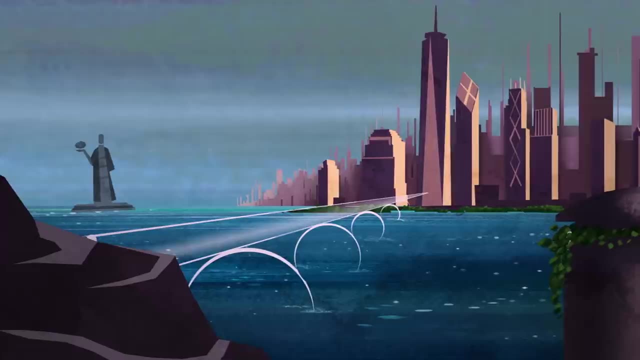 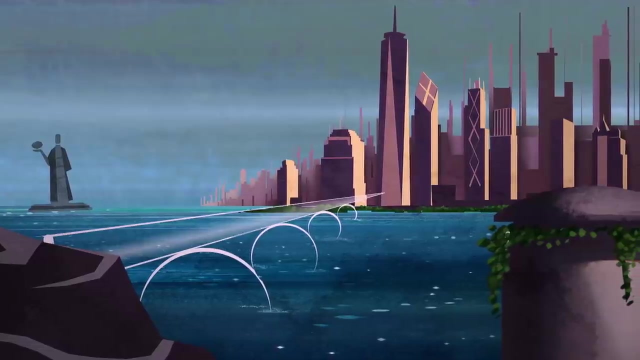 allowed cities to expand and integrate further, establishing police, fire and sanitation departments, as well as road networks and, later, electricity distribution. So what is the future of cities? Global population is currently more than 7 billion and is predicted to top out around 10 billion. 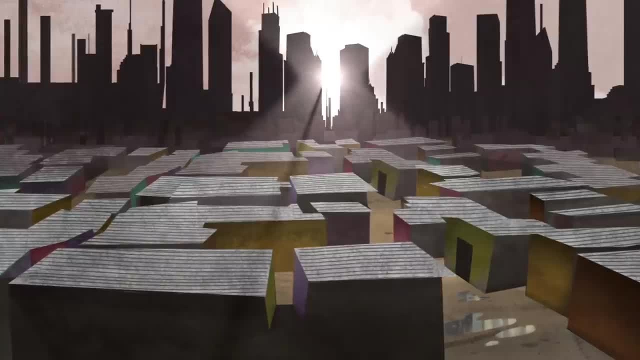 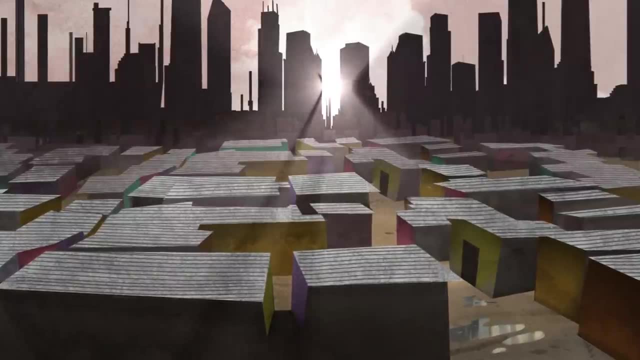 Most of this growth will occur in the urban areas of the world's poorest countries. So how will cities need to change to accommodate this growth? First, the world will need to seek ways to provide adequate food, sanitation and education for all people. 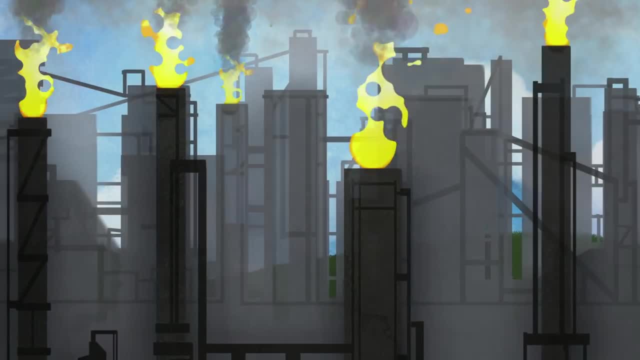 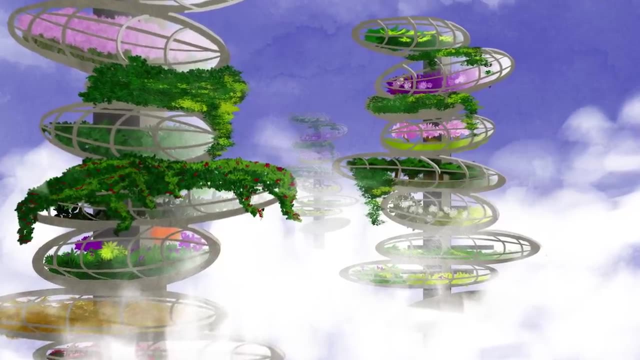 Second, growth will need to happen in a way that does not damage the land that provides us with the goods and services that support the human population. Food production might move to vertical farms and skyscrapers, rooftop gardens or vacant lots in city centers. 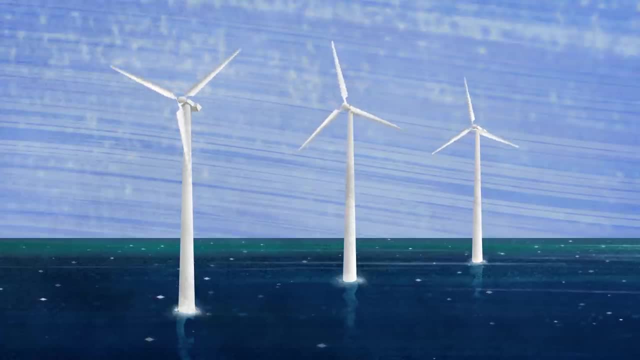 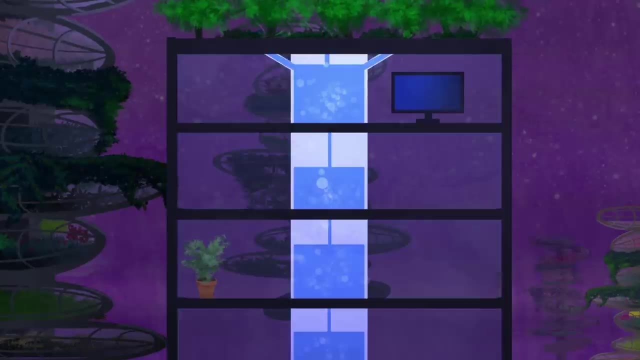 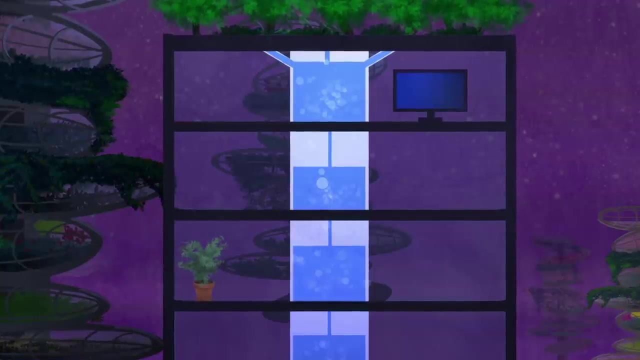 while power will increasingly come from multiple sources of renewable energy. Instead of single-family homes, more residences will be built vertically. We may see buildings that contain everything that people need for their daily life, as well as smaller, self-sufficient cities focused on local and sustainable production. 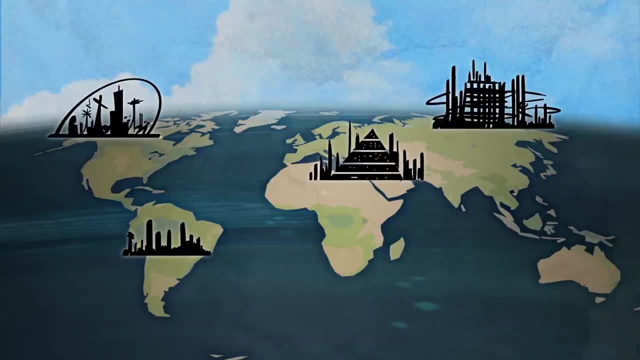 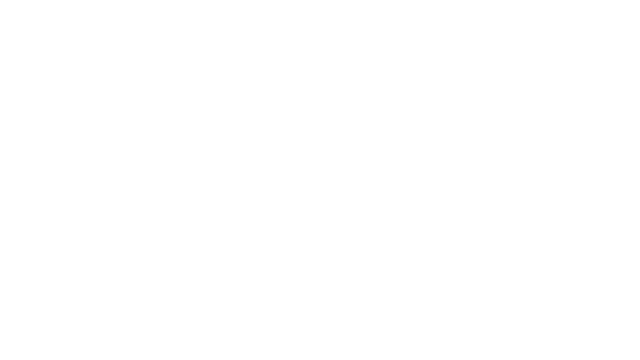 The future of cities is diverse, malleable and creative, no longer built around a single industry but reflecting an increasingly connected and global world. Subtitles by the Amaraorg community.